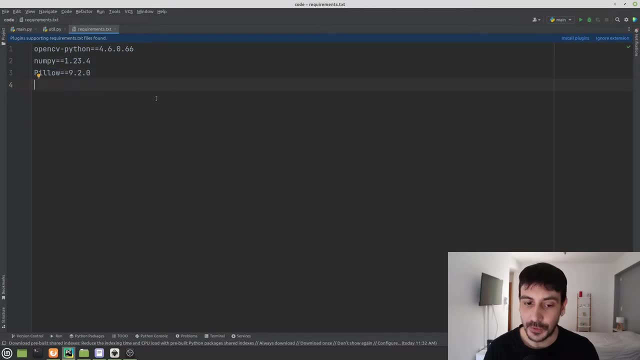 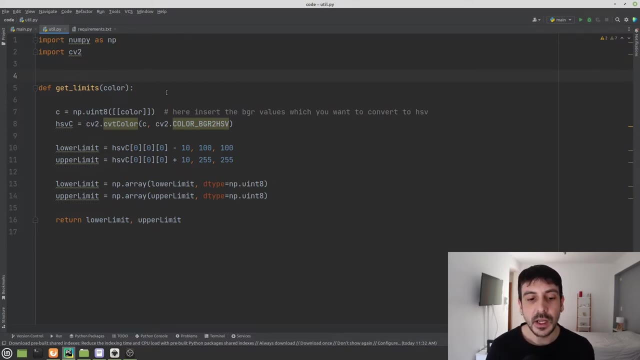 to install all these dependencies. before starting this tutorial, let me show you a file i have created and that's going to be super, super useful for today's tutorial. i have created this utils file. it's called utilepi and it contains a function, only one function. 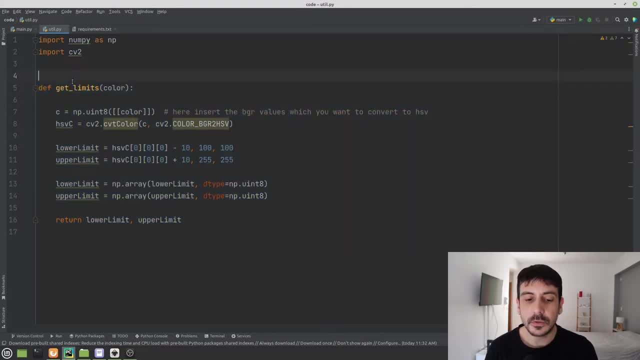 and this function is going to be super, super, super, super useful. later on on this tutorial, you are going to see exactly why. as this is a tutorial about how to detect color using python and opencv, you can see that the input of this function is exactly that: it's exactly a color. so 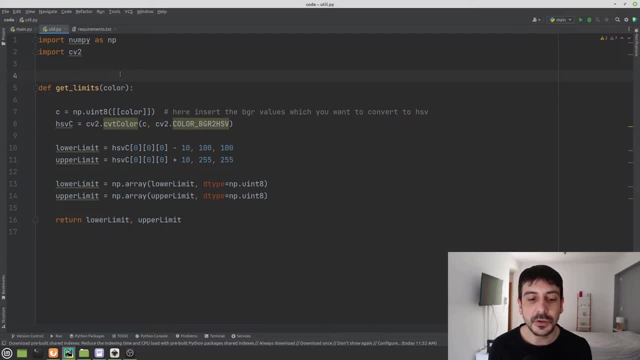 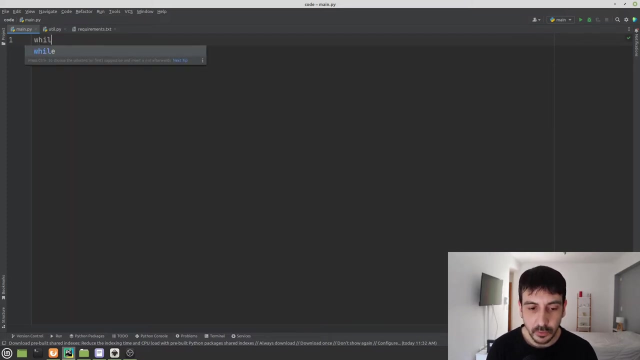 this is going to take care of some parts of our process, which is going to make everything much, much simpler and much easier for us, but you're going to see exactly why in a few minutes. now let's start with this tutorial and the first thing i'm going to do is to load, or my webcam, because we are 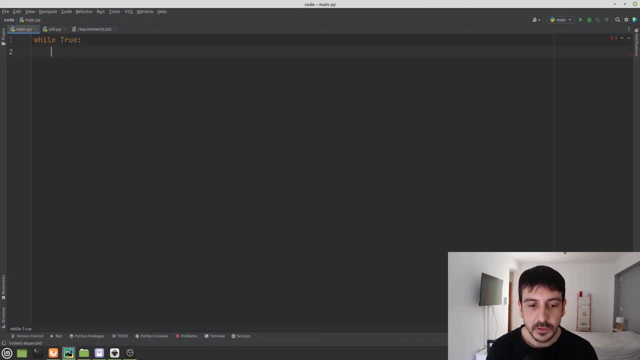 going to work a lot with the webcam today, so i'm going to create a while through and i'm going to say something like: i need to import cv2. then i'm going to create an object which is cap and this is going to be cv2 video capture and i need to specify what's the webcam i want to load using. 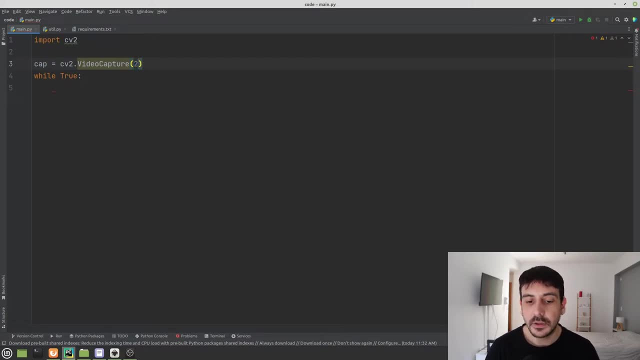 opencv and i'm going to specify what's the webcam i want to load using opencv. and i'm going to specify: it's the number two. this is going to depend on how many webcams you have, uh, connected to your computer. it may be the number two, one, zero, um, who knows if you, if you only have one webcam, it's most. 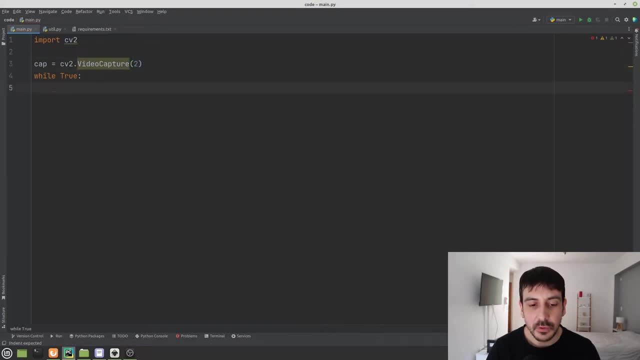 likely the number zero, but in my case i'm going to use number two. so well, true, i'm going to read frames for from my webcam, so this is going to be something like capread, and then i'm going to visualize this frame. so i'm going to use this frame, and then i'm going to use this frame. so 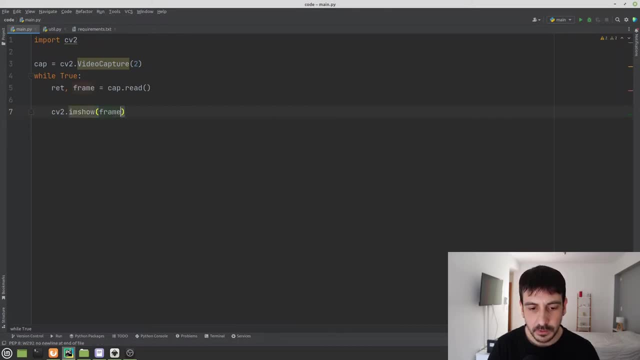 i am calling to imshow frame and i'm going to call this window frame, so that's pretty much all. then i need to close this window and i'm going to do it once i press the letter q. that's going to be all, and then i'm going to release memory and cv2, destroy, sorry, destroy all windows. 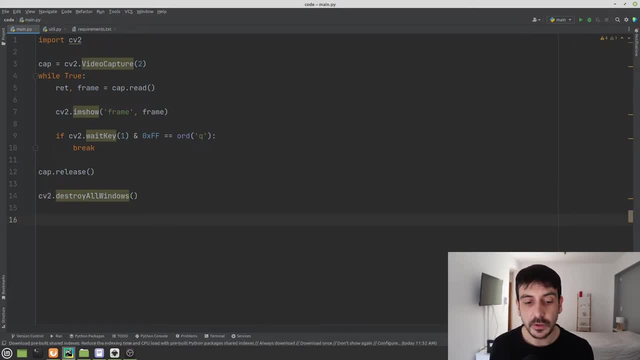 okay, this is the end of this video. i hope you enjoyed it. if you liked it, please subscribe and leave a like if you want to see more videos like this, and i'll see you in the next video. bye, bye. the most basic structure we need in order to do nothing, in order to open our webcam and just 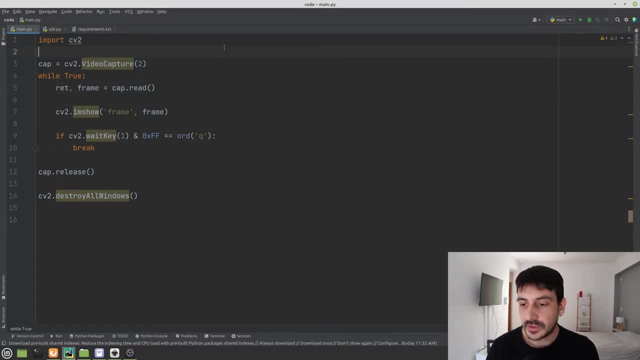 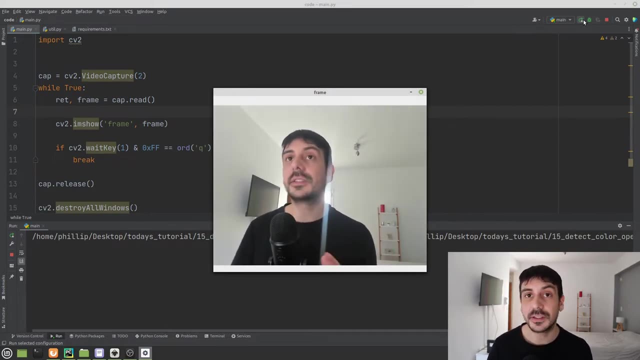 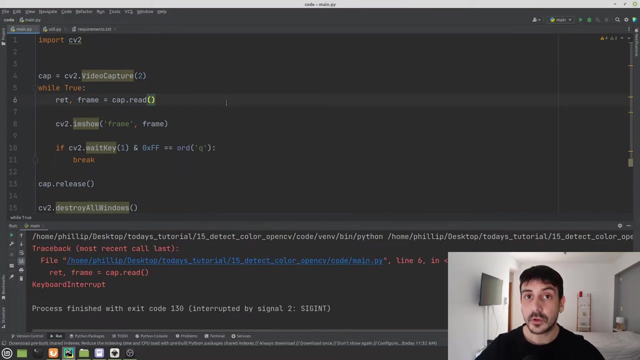 visualize our webcam stream, and i am going to press play to see exactly how this looks like, and you can see that we, so far, we have absolutely nothing. we are only visualizing my webcam. okay, so let's continue, uh, what i'm going to do now. we have built our most basic structure. 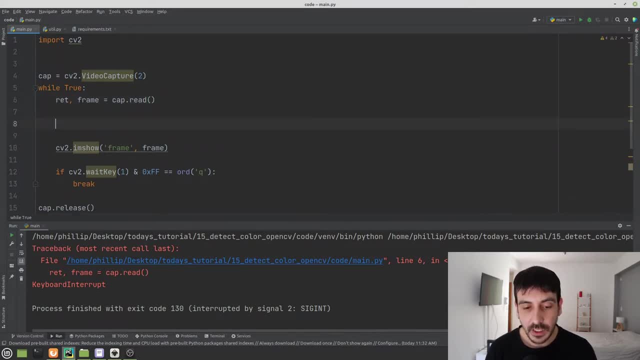 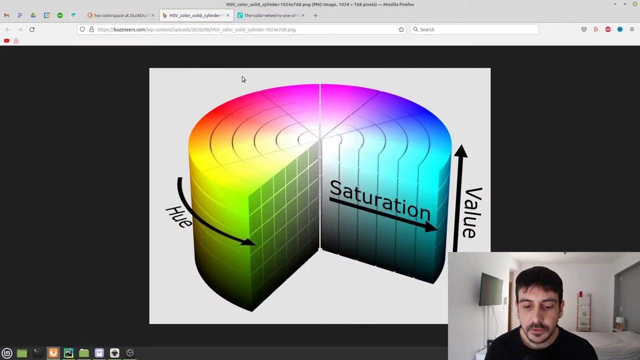 in order to visualize our webcam. now let's, let's handle all the color detection, which is what we are going to do in today's tutorial, and before starting the coding, then the sentences, all the code we need in order to detect color, i'm going to give you, like a very quick instruction in 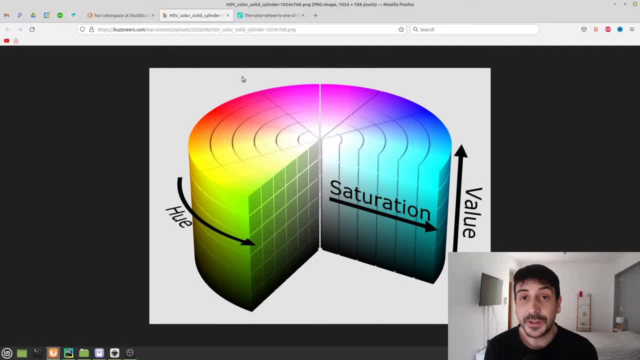 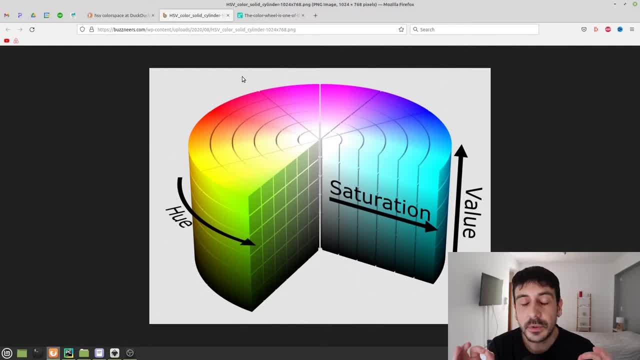 blue, green and red colors. absolutely every single pixel, absolutely every single color in our image can be expressed as a combination of these three colors: blue, green and red. but in some cases it's going to be very convenient to convert or representation to convert or image or color space. 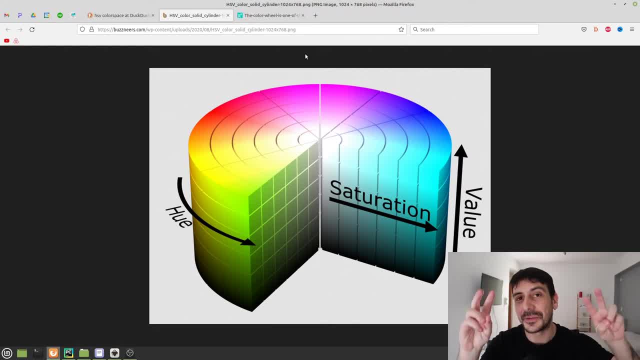 from vgr, which is the original representation or the original color space, into a more convenient color space, depending on our use case, depending on what we want to do with our images, and if we talk about detecting colors, we are going to work with the hsb color space. this is an image of how the hsb color space looks like, or this is like a model. 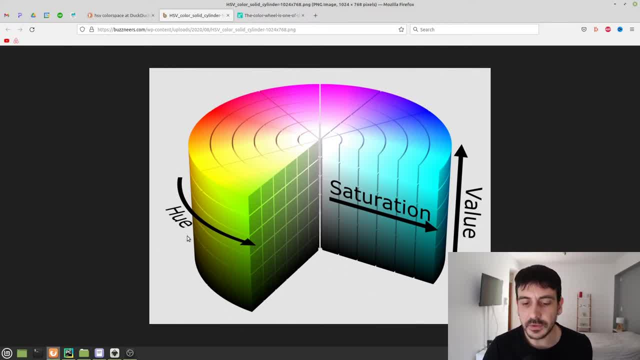 for the hsb color space and you can see that we have something that looks like a cylinder and we have three different channels or three different components in this cylinder. they're called hue, saturation and value. and yeah, i'm not going to show you the hsb color space, but 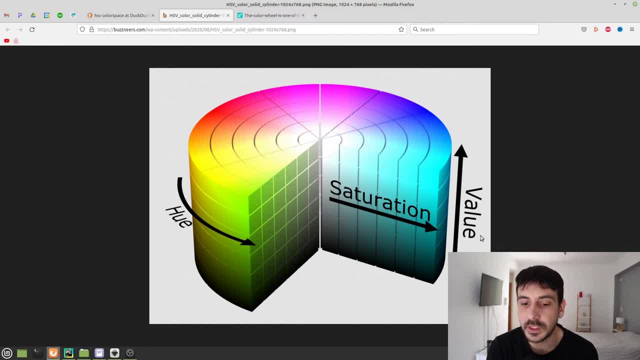 i'm going to give you like a very comprehensive description of this color space, because we don't really need to know super, super in detail what exactly is the value, what exactly is the saturation. we don't really need to know like super, super comprehensively about these things, but we are. 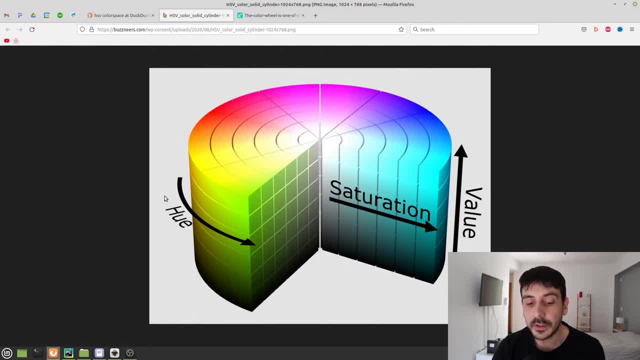 going to work mostly with the hue channel and if we look at the hue channel, this is where we are going to have our information related to the color of our image, to the color of all the different colors. we are going to be looking at a cylinder which contains information for hue saturation and 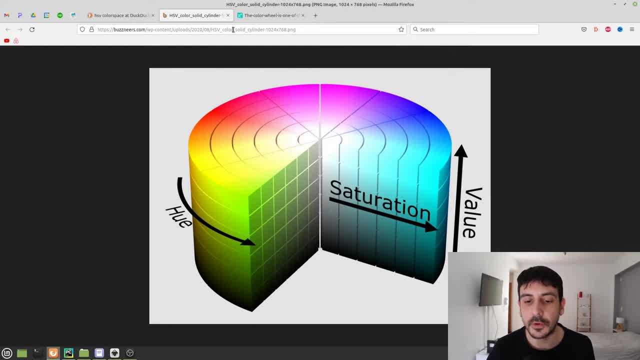 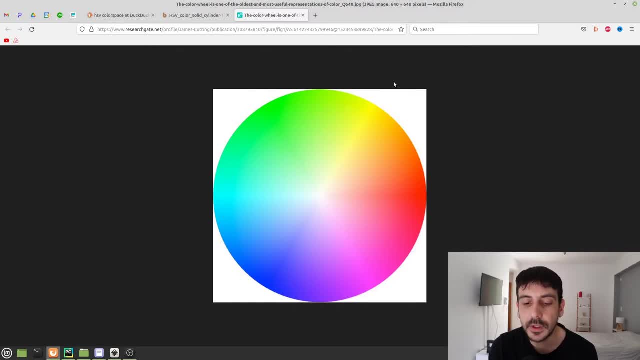 value. but let me show you how this cylinder looks like if we look it from above. if we look at this cylinder from above, we are going to see something like this. so this is what i want you to think about when we think about the hue channel: that we are going to have something like a circle and, as 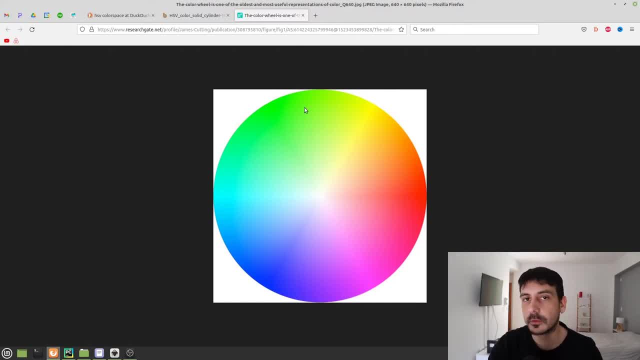 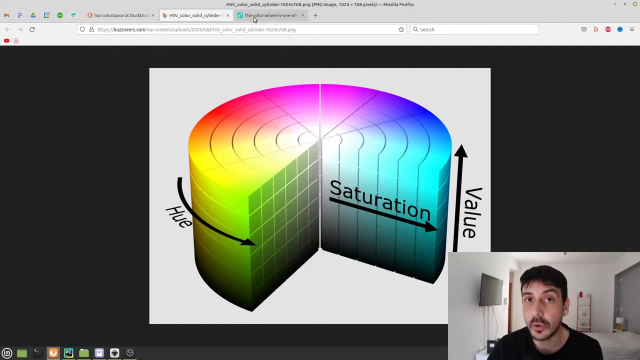 we go through this circle, we are going to be changing, like through different colors- so different- to have different values in this hue channel. that's pretty much the intuition behind working with the hsb color space. the information related to the image color, to the pixels colors, is going. 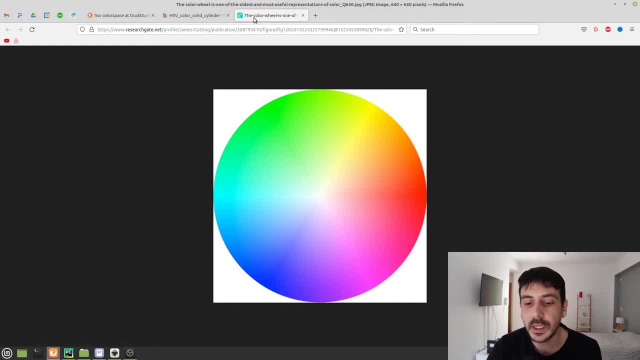 to be encoded in the hue channel. right, we are going to use this information in order to detect an image, color, pixels, colors, and we are going to tell python, we are going to tell our program or software to detect all pixels from a given color. so, for example, i have already shown you that we are going to detect the color yellow, so we are. 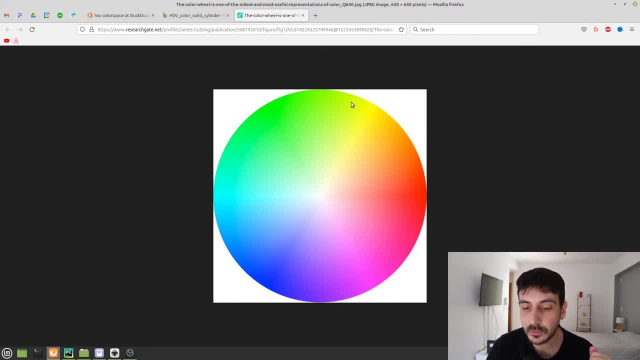 going to tell this software to give us all the pixels within this region, which is the yellow region. now, we cannot ask this program to give us only one value for the yellow color, because you can see that this is like an entire region, right, there is like an entire region of the hue component. 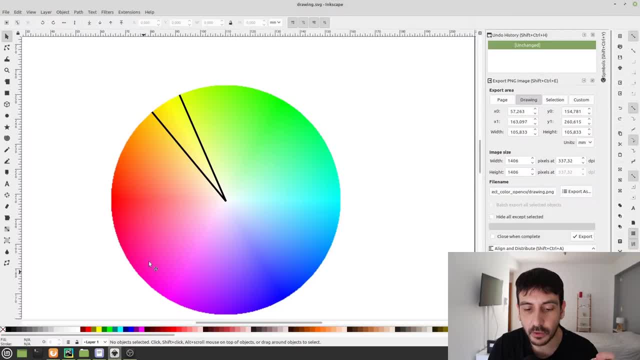 where we have yellow. so what we are going to tell our program and what we are going to be coding today is defining something like an interval, something like a region, something like like this, where we are going to define what's the color we are interested in and, for example, in our case, we 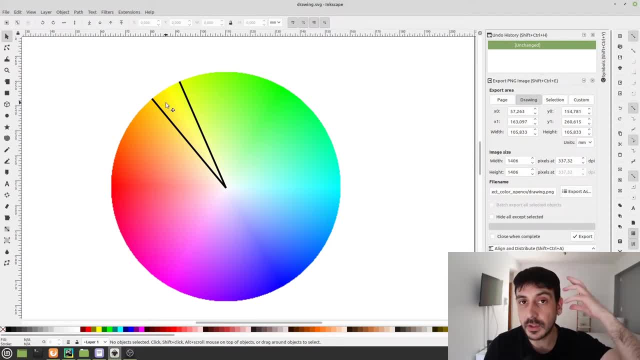 are going to work with yellow and if you think about this representation, if this is something, that, if this is our model for the color, for the hsb color space and for the hue channel, you can see that, in order to specify the yellow, in order to tell python to give us all the yellow pixels, 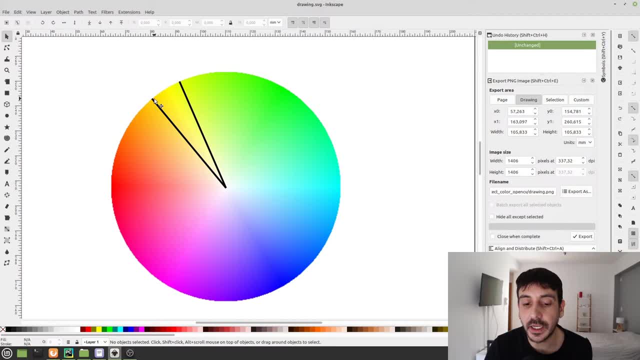 we will need to specify something like two inter, like an interval, something like these two values. we are going to tell our program to give us all the pixels that are within this interval. we are going to specify two values and then we are going to tell the software we are going to 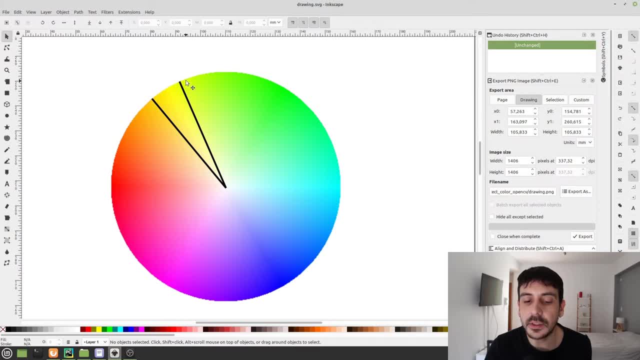 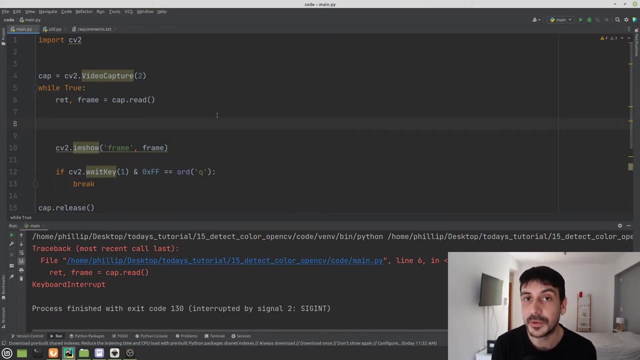 code today to give us absolutely all the pixels that are within these two values. pretty much the idea what we are going to do in today's tutorial. we are going to use the hsb color space. we are going to detect colors using the hue component, the age component, the hue channel of. 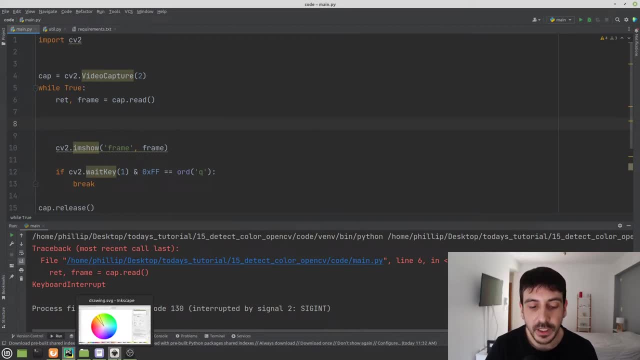 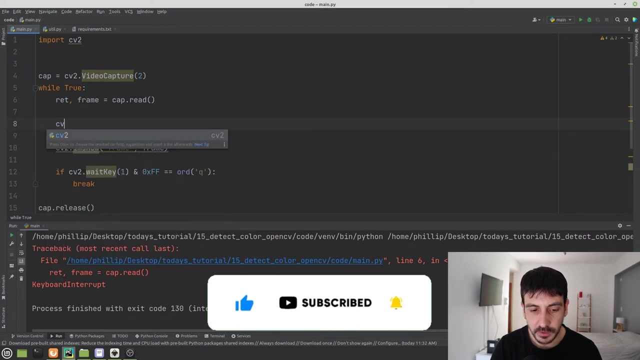 this hsb color space, and then we are going to define two values and we are going to ask our software to give us all the pixels within these two values. that's pretty much the idea, so let's see how we are going to do that. so the first thing we need to do is to convert our image from the 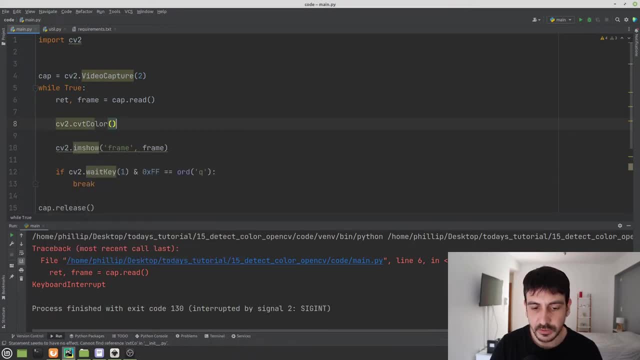 vgr color space to the rgb color space. so we are going to something like frame, then cv2 color vgr to hsb. so with this sentence we are converting our input image from the original vgr color space into hsb and this is going to be something like hsb image and that's pretty much it. so this is. 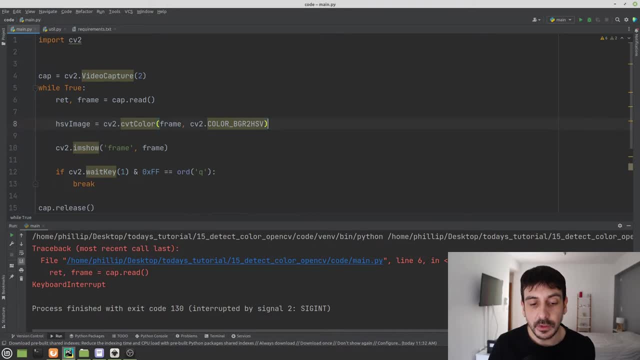 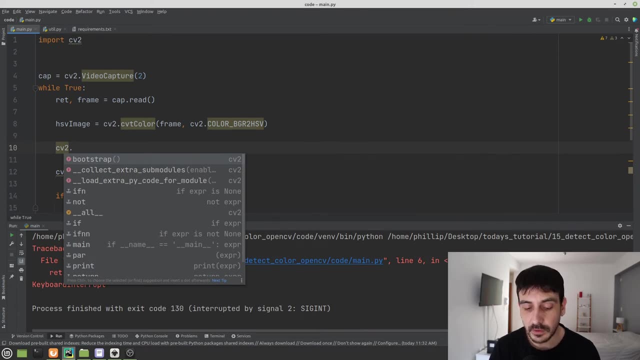 our hsb representation for image and now the. what we are going to do now is we are going to call a new opencv function, a function we have never used before, which is called ring range, and this is a function we are going to use in order to get a mask from all the pixels that belong to the color we want to detect. 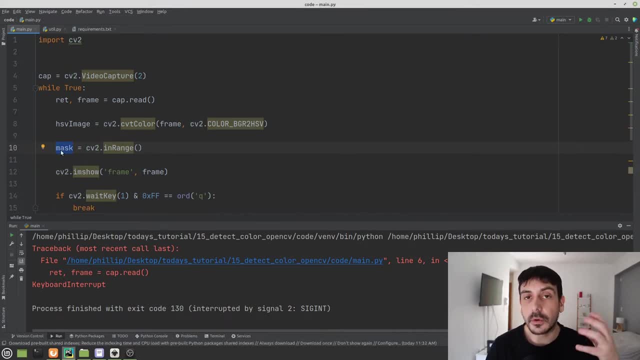 so we are going to use this function and the return from this function is going to be a mask. it's going to be the location of all the pixels containing the information we want. and the way we are going to call this function is that we are going to input hsb image and then we are going to input two. 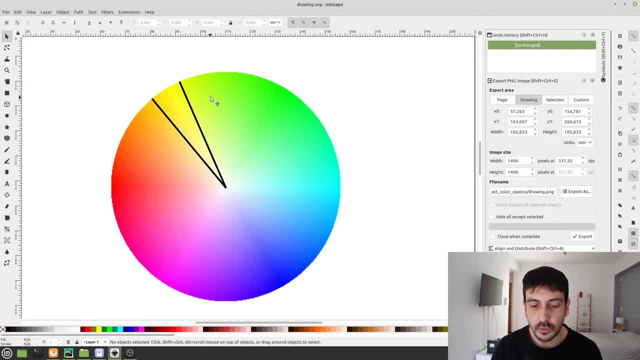 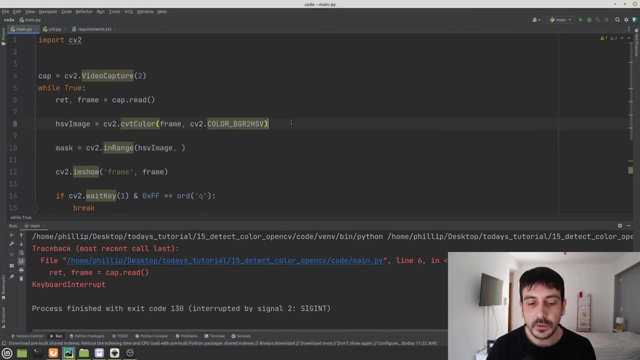 values, which are going to be exactly these two numbers, exactly the interval for which we are going to tell opencv to give us all the pixels in this image that are in between these two values. so we are going to input two values and the way we are going to 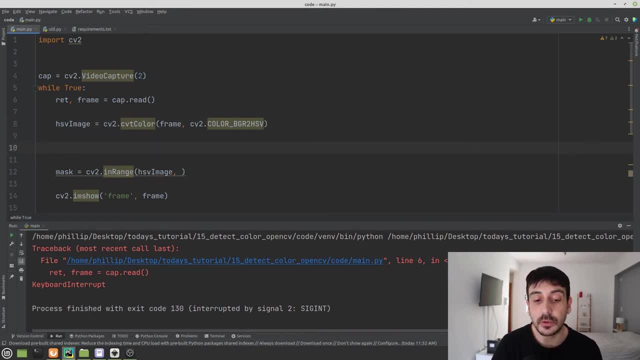 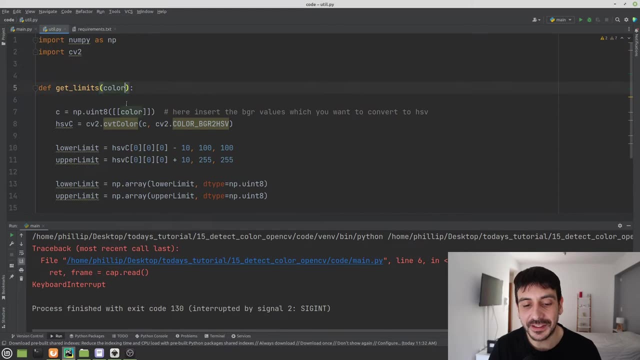 um define these two values. the way we are going to find these two values is by calling the function i have defined in the util file. so this is exactly why i have defined this function. by calling this function, it's going to be very, very simple to get exactly what is the interval we need in order to 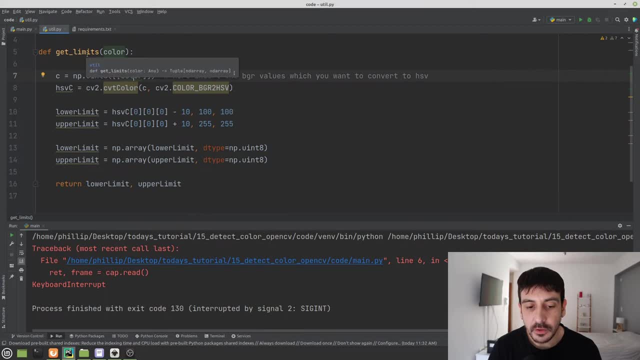 get the color we want, and you can see that for this function, the way we are going to use it is that we are going to input a color and the output is going to be exactly two values, which are named lower limit and upper limit. the way we're going to use this, i'm going to import, so i'm going to 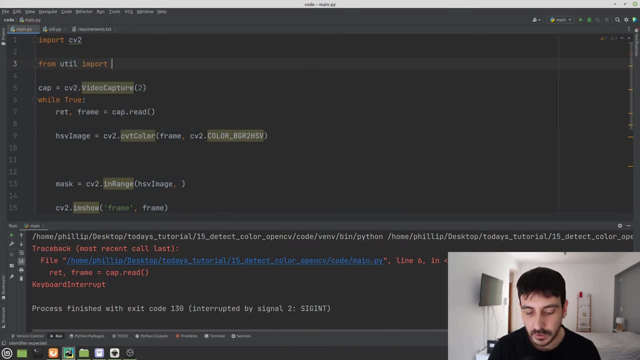 say something like: from util import, get limits and then, as you can see, here we are. we need to input a color. so i am going to define the color we are going to detect today, which is going to be called yellow, and it's going to be 0, 255, 255. this is yellow in. 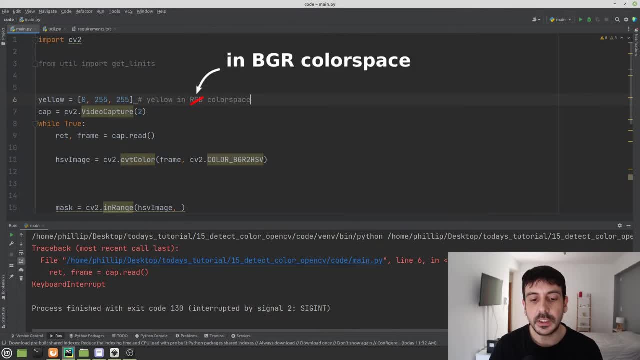 rgb color space. right, if we want to define yellow, this is exactly the value for yellow in b, g, r color space. so the way we are going to input this function is by calling get limits and then we specify the color. we can do it like this so it's more clear, and this is going to be lower limit and upper limit. 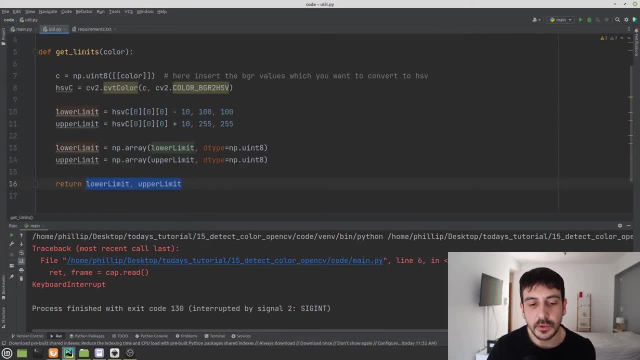 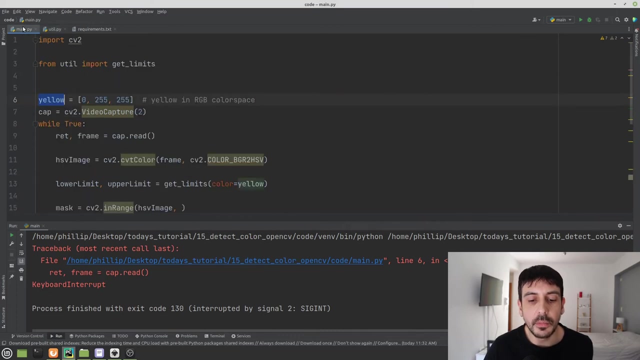 you can see that we need to specify our colors in bgr, because this function take takes care of converting this color to hsb and then it just continues to do some additional processing. but we definitely need to input this color in bgr and then this function will convert. 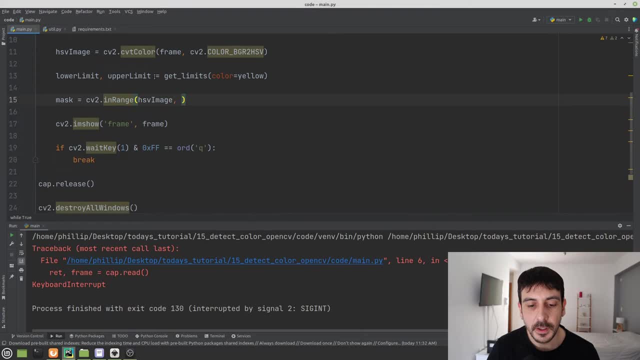 the color into hsb and we'll do some additional stuff, and now the only thing we need to do is to copy these two numbers and to paste them here. so we are taking our hsb image and these two limits and we are calling the cv2 in range function. 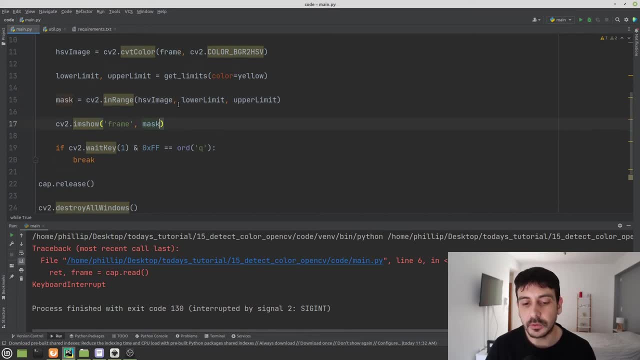 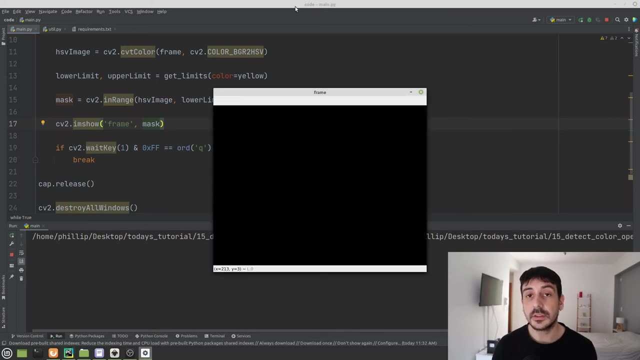 now let me show you how this mask looks like before continue with your process. maybe it's a good idea to show you how this mask looks like, so i'm just going to press play. you can see, this is a mask. this is exactly how the mask looks like, so we are looking at a. 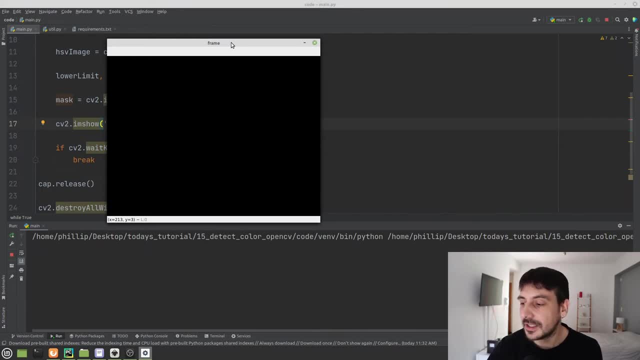 completely dark, completely empty image. but let's see what happens when i input a yellow object, so something that's completely yellow, and you see what happens. so when we talk about this mask, this is exactly how this mask looks like. we are getting all the pixels within our image that are: 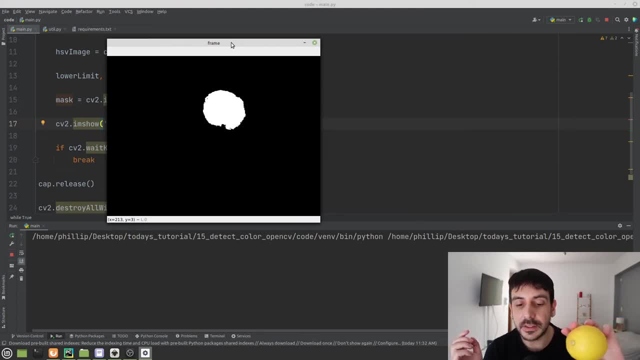 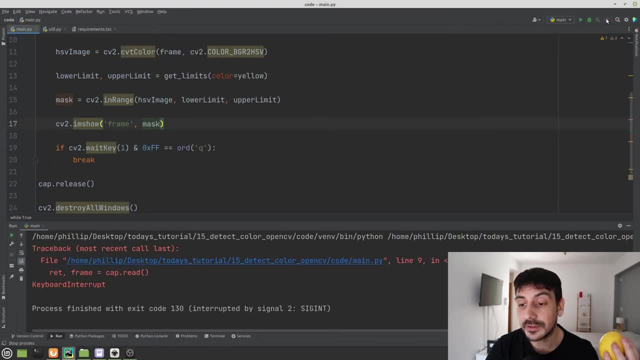 from a given color. we have specified yellow, and this is exactly what happens: we are getting all the yellow pixels in our image, okay, so now let's continue, and you can see that we are very pretty much there. we are. we have almost completed this tutorial, because the only thing we will need to do now is to draw a bounding box in our image. so, yeah, this is a 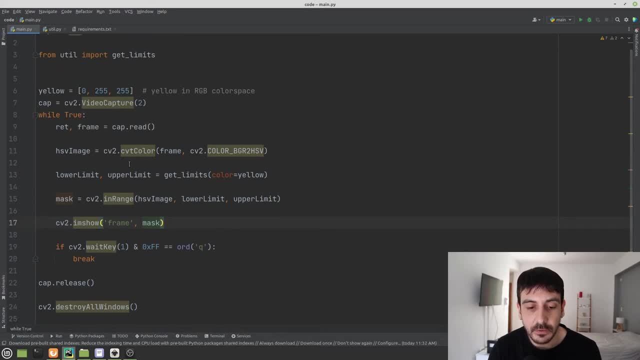 this is going to be a very short tutorial. you can see that we have only written a few sentences and we are pretty much there. we have already our mask with the location of all of all of our yellow pixels, but now we need to draw the bounding box. and not only that, but we need to detect. 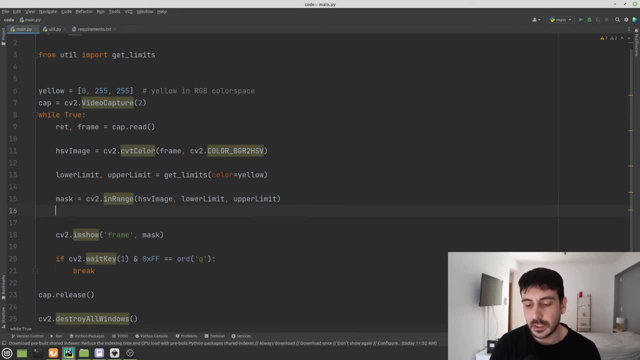 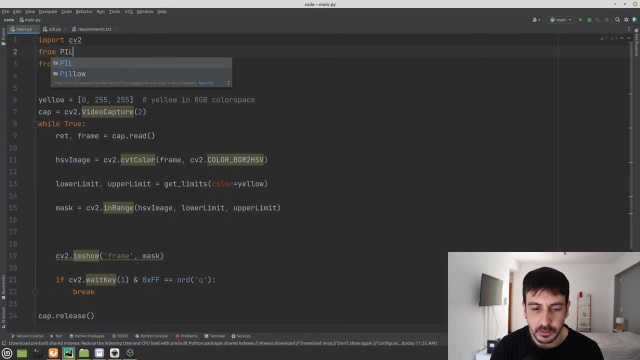 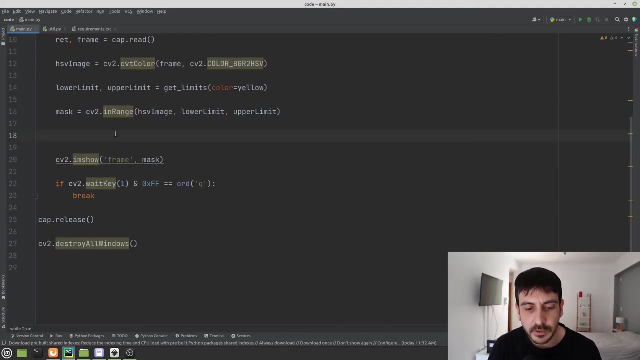 exactly what's the bounding box for all of these pixels, and this is where i am going to use the pillow library. so i'm going to from peel, i'm going to import image, which is the function we are going to use from the pillow library, and this is what 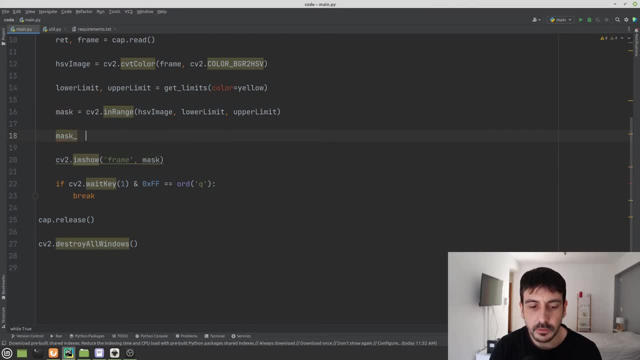 i am going to do. i am going to define a new variable which is going to be called mask underscore, and this is going to be image from array and i'm going to input my mask. so this is a new variable which is called mask underscore, and the way we have created our image is taking our 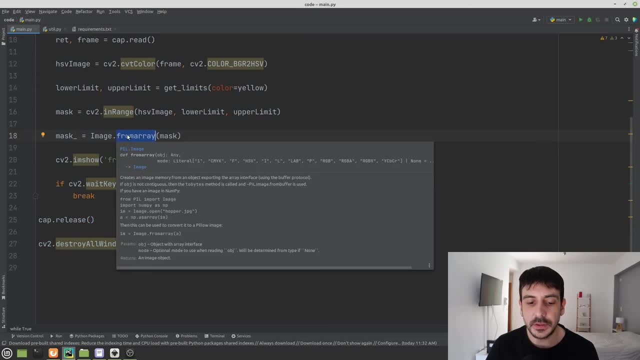 mask and then calling image dot from array. so this is basically the. the only thing we are doing is converting our image from being an amp- your right, which is opencv representation for our image, and we are just converting this image into pillow. that's the only thing we are doing. we are keeping 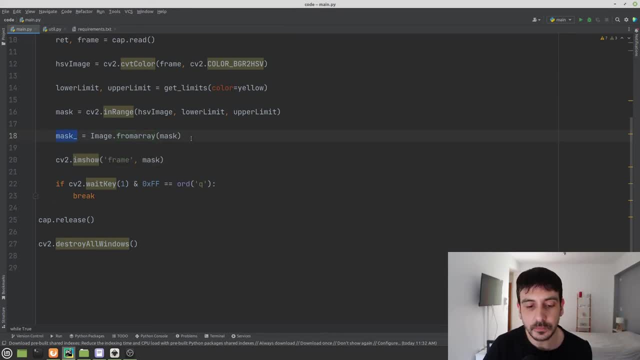 exactly the same information, but in a slightly different format. so what you'll see is that we are actually making it into a mask, because we are making the connection part of our image. we are making our image into a mask which is called MAYOR. so what we are doing is that we are making this conversion is because we are going to call. 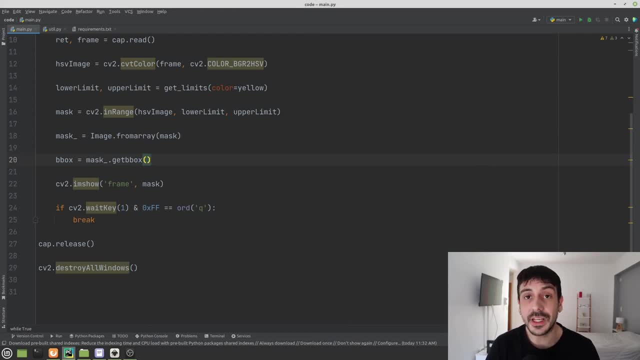 a function from this new variable which is going to be get bounding box, and that is it. if we want the bounding box of all of our yellow pixels, if we want the bounding box of the mask, the bounding box we need for our object, this is exactly why we are using pillow. 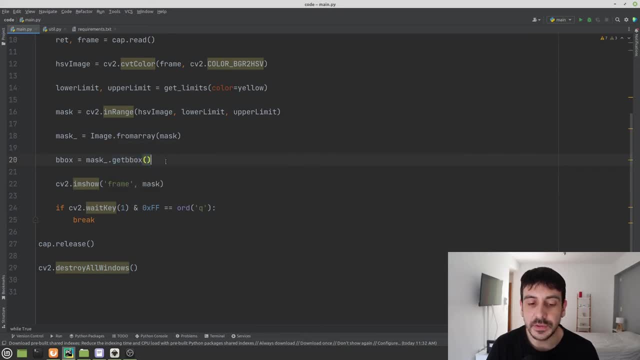 in order to get the bounding box, because it's going to be super, super easy to do it. okay, and now the another thing I can show you is how the bounding box looks like when we have detected an object and when we have not detected absolutely any object. so I am going to print bounding box and I am going to press play again. 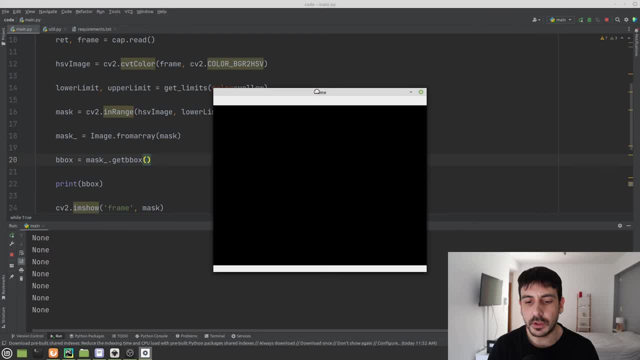 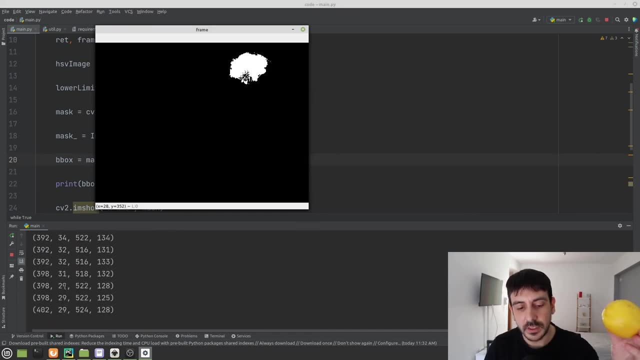 you can see now there's not any yellow object in our image, so nothing happens and bounding box is none. and let's see what happens when there is an object. you can see now we are getting some numbers and these numbers are exactly the bounding box, and if there is not any object, I get none. so what I am going to? 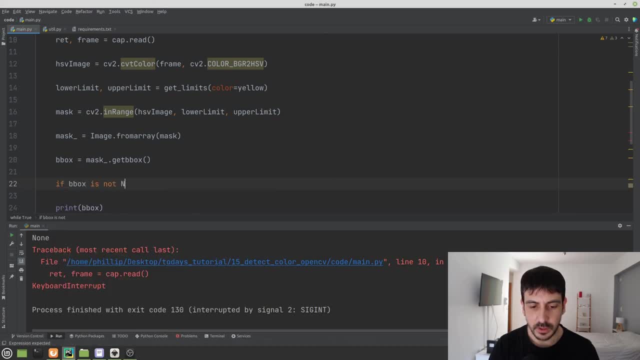 do is, if bounding box is not none, then I am going to get the locations, I'm going to unwrap my bounding box, which is going to be something like this, and then I am going to draw a rectangle with this bonding box. on the rectangle will be something like this: 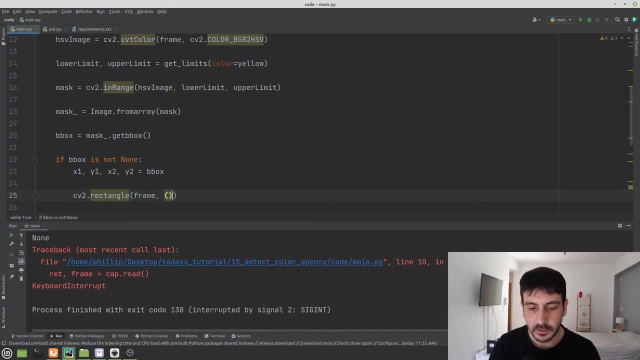 let's draw the rectangle on the original frame. then we need to specify the upper left corner, which is X1, Y1, then the bottom right, which is X2, Y2.. then the colors, which Let's draw this bounding box in green, and then the thickness which I'm going to specify: 5. 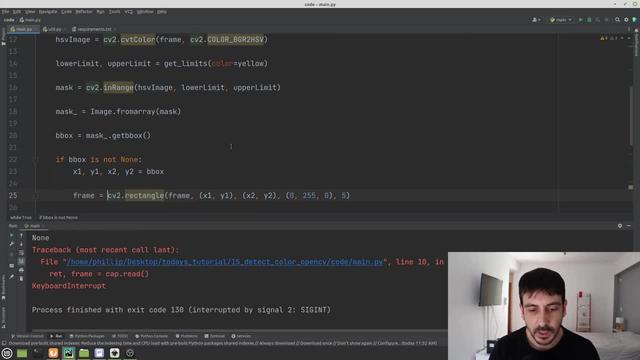 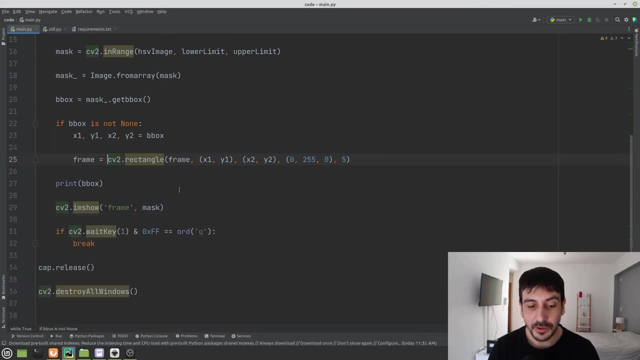 and this is going to be equal to our frame, and That is it. That is all. If I press play now, we are going to see our image, we are going to see the Stream from our webcam and we are going to see the bounding box drawn on top of this. 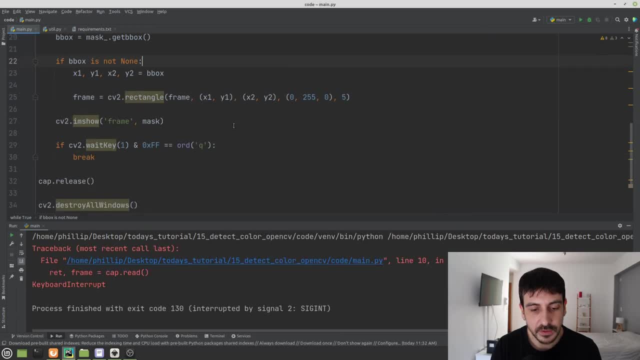 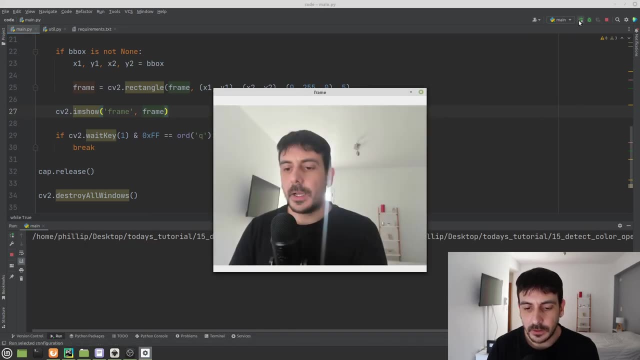 Webcam. so, for example, Here I'm still drawing the mask, I'm going to draw the frame and I'm going to press play again And you can see, this is me. There's not any yellow object, So nothing is going on, and this is what happens when I have a lemon or which is a yellow object. 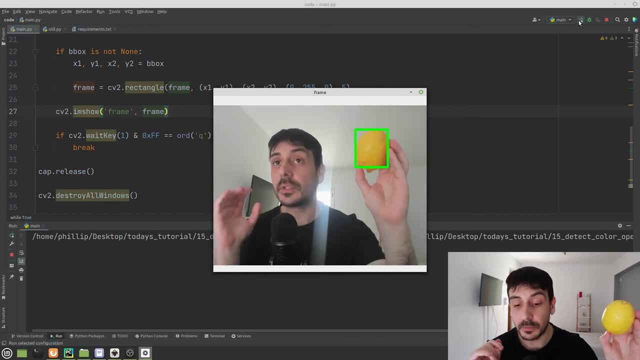 You can see, we have at the exact location, the exact bounding box for this object. So, yeah, this is pretty much all. this is pretty much the idea for Today's tutorial, and I'm not sure how many frames per seconds we are getting, but you can see that this is pretty, pretty real-time. 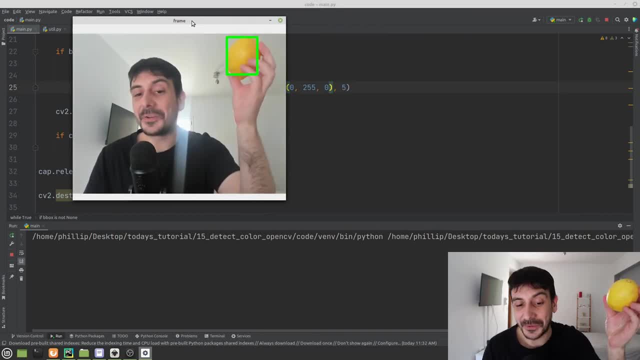 I mean, we are getting a lot of frames per second. we are definitely getting a very, very good detection, a very fast detection, and We are getting a very good resolution. and, most importantly, we are not using a GPU. We are running this script on a CPU and you can see how good of a detection we have. also, if I use another. 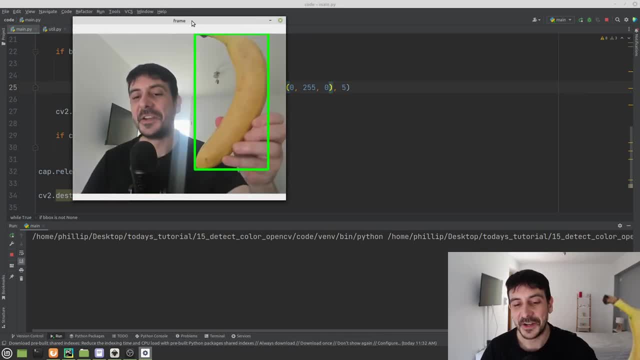 Another yellow object, for example a banana. You can see that we are getting a very good detection as well. We are detecting exactly where the banana is located. Yeah, so we are detecting the yellow color very, very accurately. We are doing it very, very fast and we are not using a GPU, So this is amazing. 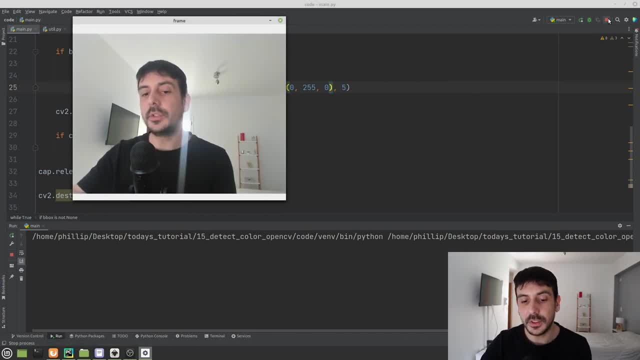 This is a very, very good object detector. So this is going to be all for this tutorial, and this is exactly how you can detect color using Python and OpenCVD. Please let me know in the comments below What do you think about this video, and please let me know if you have any idea of some very cool and awesome project. 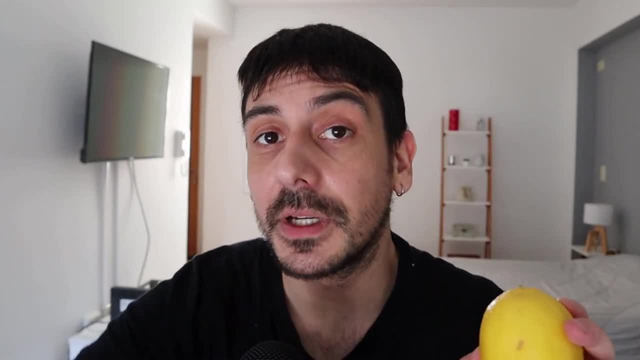 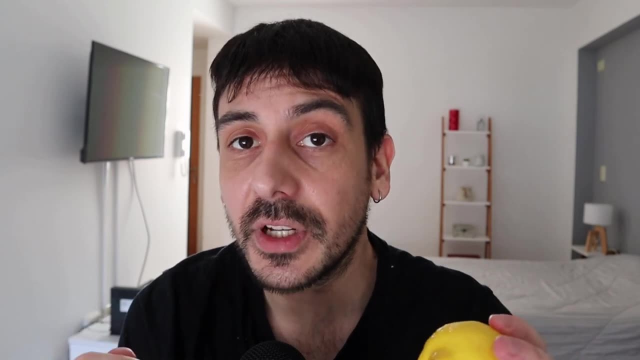 We could work on this channel. So if you enjoyed this video, I invite you to click the like button, and I also invite you to subscribe to my channel. My name is Felipe. I'm a computer vision developer and this channel I make tutorials exactly like this one, where I show you different applications and different use cases of computer vision. 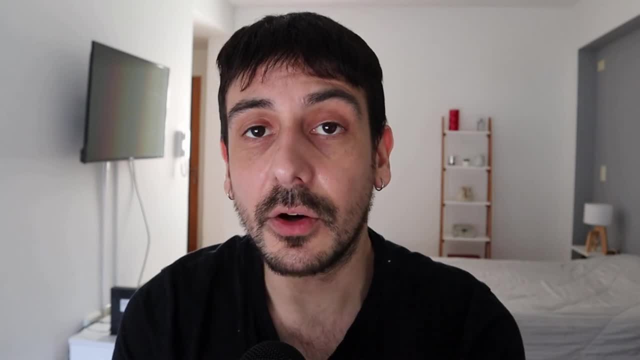 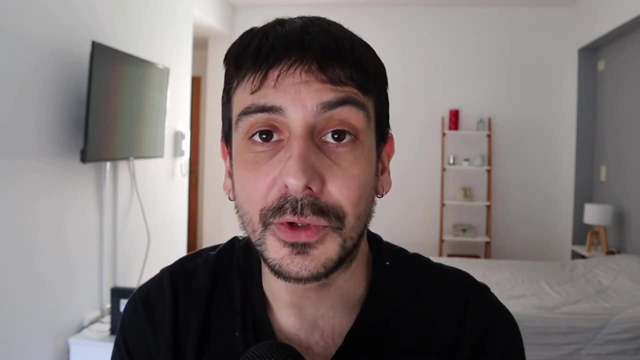 and I also share my experience and I share my resources as a Computer vision developer. So if those are the type of videos you are into, I invite you to subscribe to my channel. This is going to be all for today and see you on the next video.